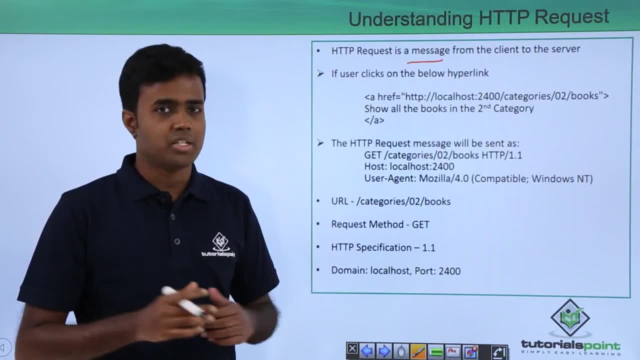 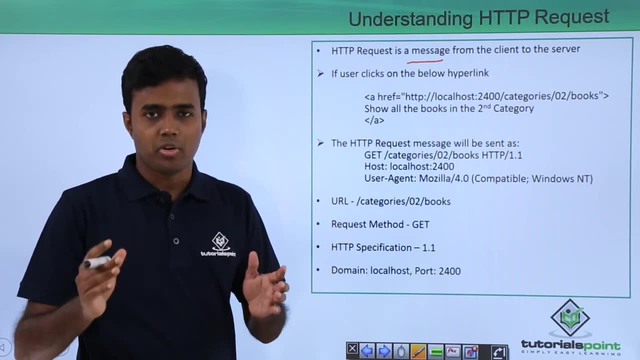 in the form of a HTTP message. And why it is called an HTTP message? That's because we are going to send the message through the HTTP protocol. And what is a protocol? A protocol is nothing but a language of communication between two people, For example, two French. 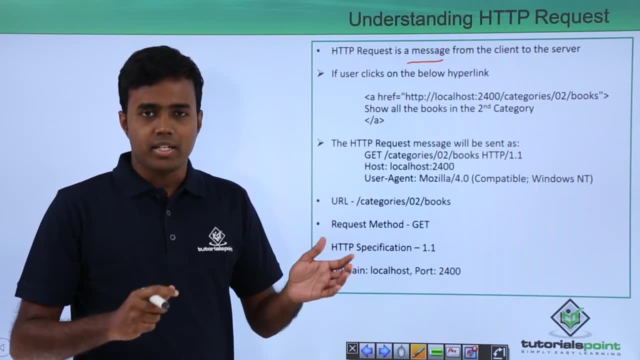 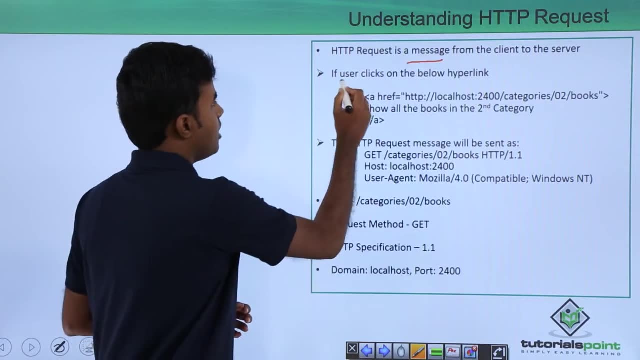 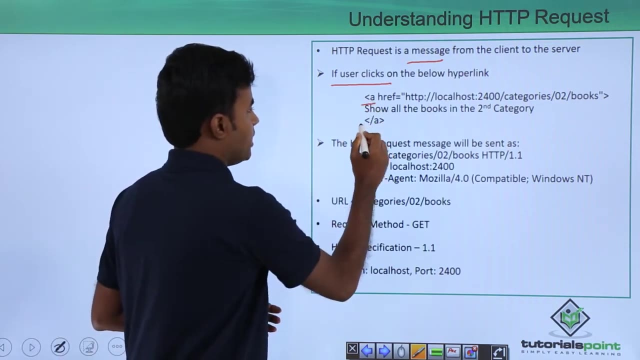 people communicate in French. In the same way, a client and a server communicate in a protocol called HTTP protocol. Now what happens when a user clicks on the Below hyperlink? In the world of web we have things called hyperlinks in the sense that the documents 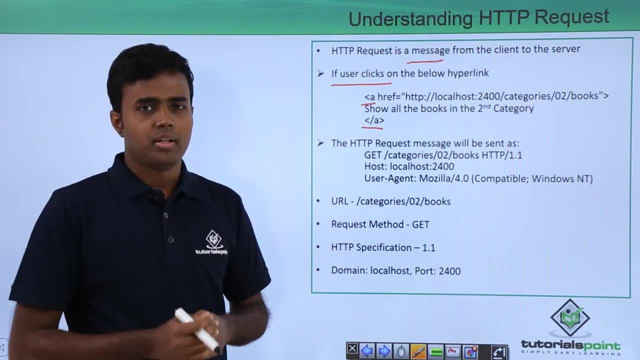 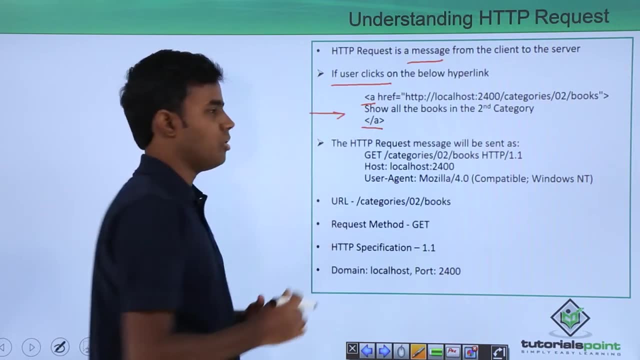 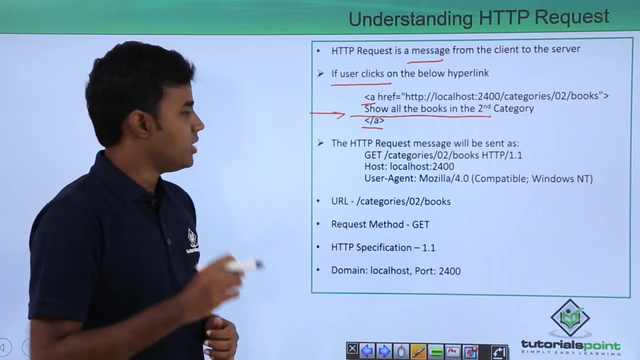 are connected to each other in the form of a hyperlink. Clicking one hyperlink leads you to another document. So suppose the user is at your homepage and is clicking this particular link saying show all the books in the second category. so what actually happens is underneath an http request. 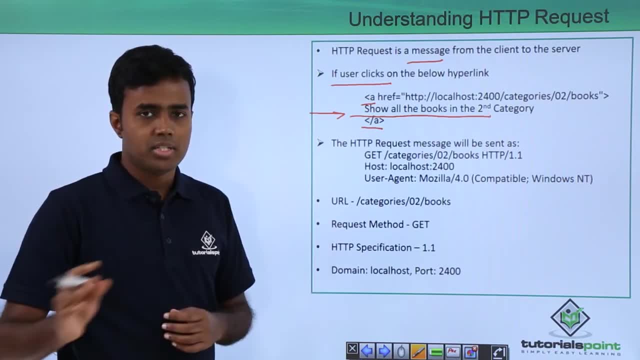 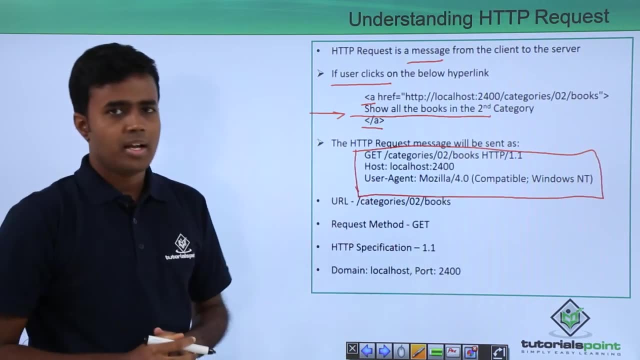 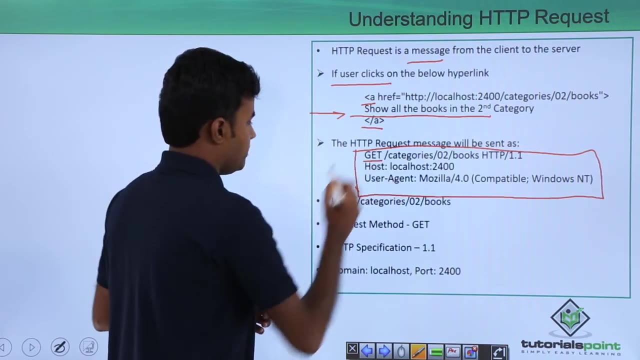 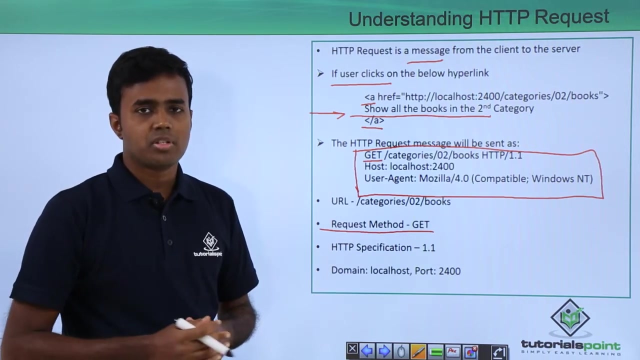 message gets sent from the client to the server, and the http request message is nothing but this. so let us break down and understand what this message looks like. over here you have something called get, which is nothing but the http request method. you have several other request methods like post put, delete, patch and so on. so get symbolizes that. 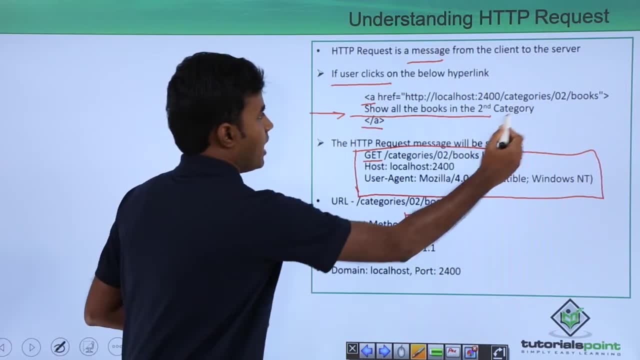 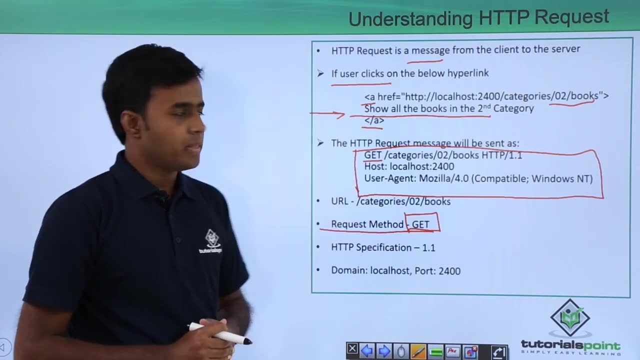 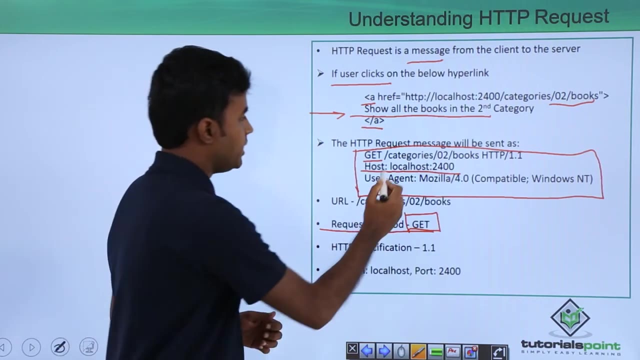 i need to get the resource that is available at this particular location. so basically, i need to get the book which is available in the second category. okay, the next thing is the host and the protocol, so this could be anything like, for example, googlecom or microsoftcom. 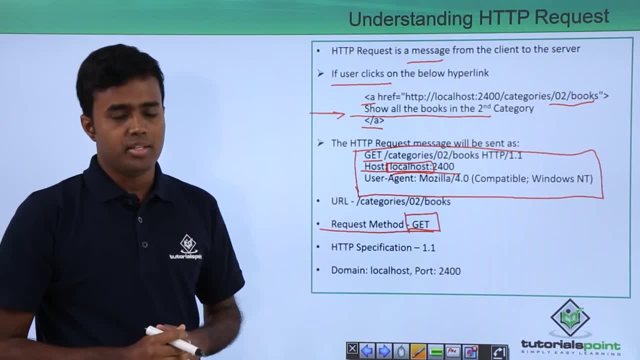 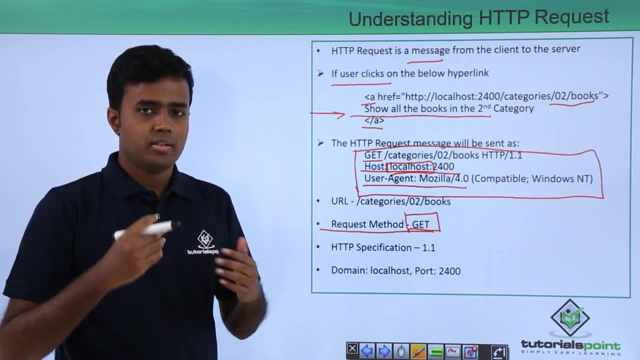 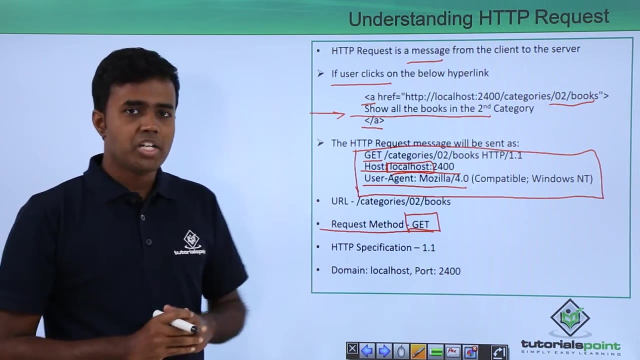 and this is the port at which that particular application is running. and the third thing is nothing but the user agent. it gives information about the operating system that you are running or the client is running and the browser that the client is using. so these give additional information to the server before processing your request. and it also gives information about